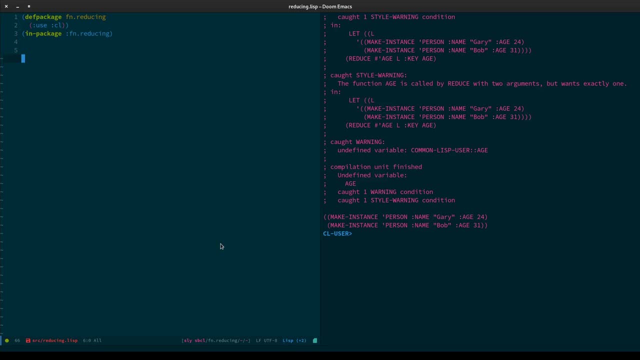 to this as folding, But all we are doing is we are taking a list Of items and we are turning that into a single value, which is not nearly as complicated as it may first appear. I know junior engineers I've worked with have found this to be the 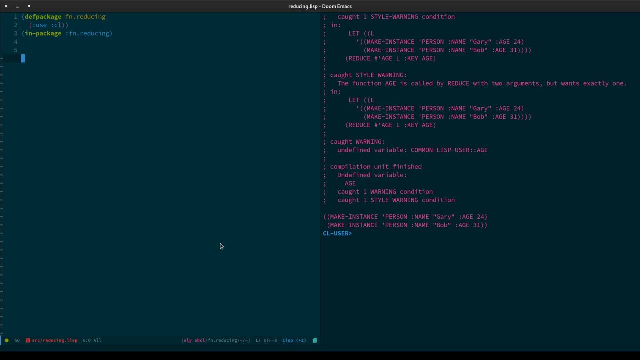 most mystifying of them all. So, with any luck, what we're going to do here is we are going to demystify this a little bit. So the first thing that we can do is perhaps have a look at the most trivial items. For example, we can take a list and add all the elements together using the plus operator. 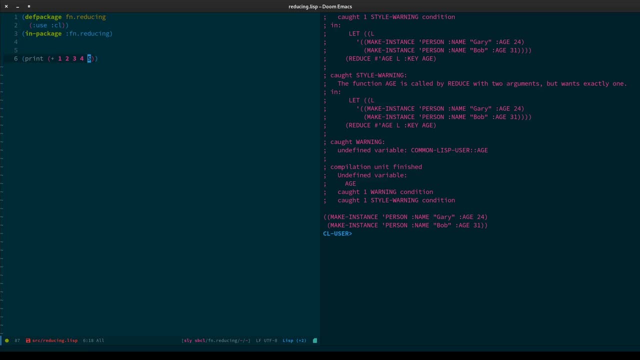 This is what it might look like if we were using Common Lisp itself, Just using the sum function, Common Lisp, the mathematical operators, the functions. here We're going to have a list of all the things. We're going to take the first three as well. So we're going to take 是, and then simply. 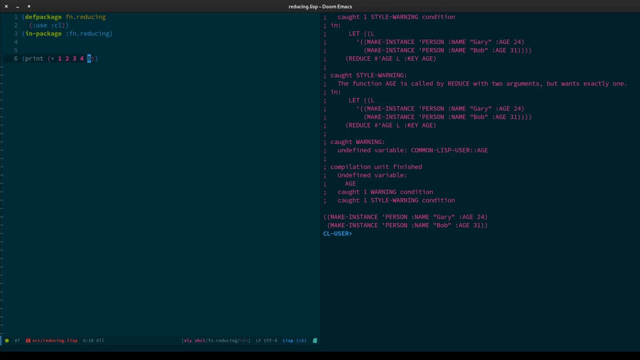 add the last key. We're going to add them together in order to make it the most simple way. Then we're going to take the last clean item. This is the one that you do: the Authentic and the денal statement. These are all the points to do in the application. 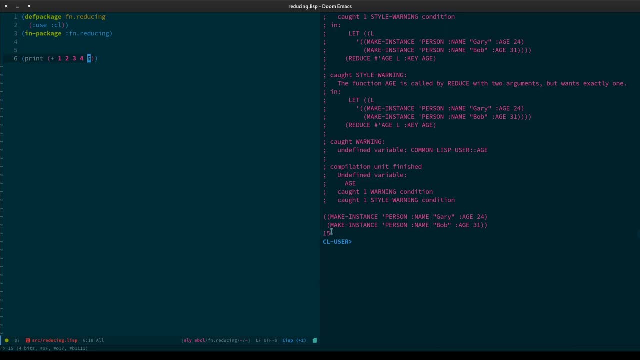 We're going to considerationally think of these as columns. We see that we're going to take the top and then the bottom. These are the columns we're going to consider as columns. You can think of the bottom as a column. Then we're going to consider the down column and the down column. 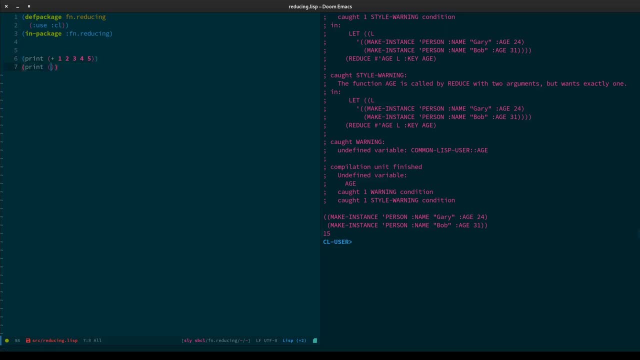 This is the bottom column. We're going to consider the bottom column. There's a list here, but that's another boring thing. But if we wanted to, so here we have the reduce function and we pass in the function that we're going to reduce everything by which, in this case, is the plus function, and then 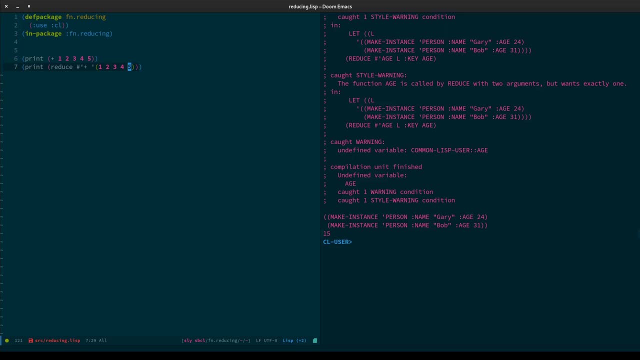 we pass in our list of 1,, 2,, 3,, 4, and 5, and that gives us the 15 that we were looking at. so let's see, let's try this with. sorry, I think I hit the desk with something. let's. 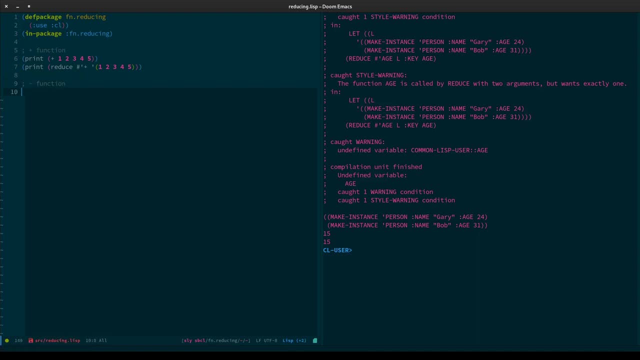 try this with a minus operator again in common lists. we could just use the minus function and we get minus 13, and the reduce equivalent is exactly the same. so we get minus 13 with that. now it's worth pointing out that reduce the order of operators in subtract matters. 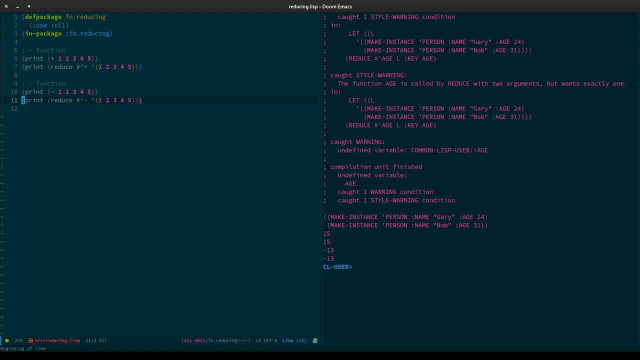 so this is not the same as this, except it is. that's interesting. there we go, so there we go. so when we have a look at subtract, we get the order of subtracting matters. so we're going to start from the inside with 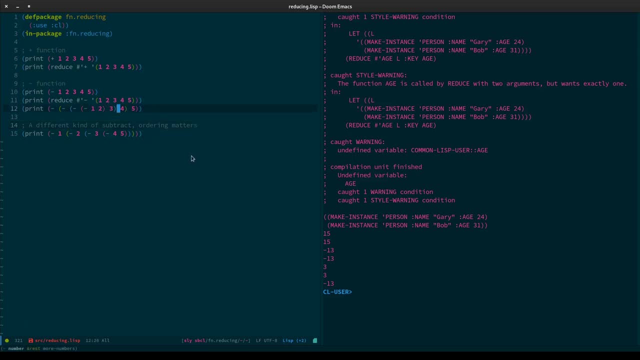 1 minus 2, and so we get to minus 13,. so these three lines are equivalent, so we get minus 1,. what we have here is we're starting with the inside out, so we go 4 minus 5,, which is: 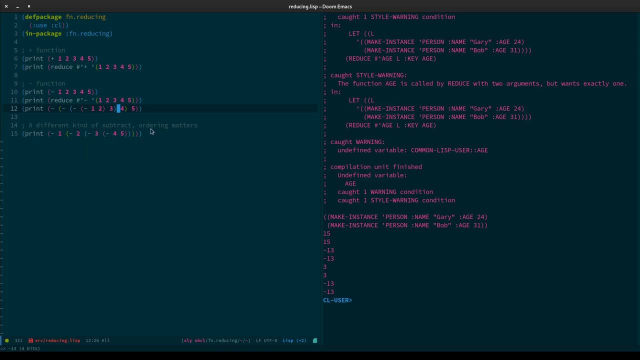 minus 1, and we get to 3,. I'm not entirely sure how the math works out. the mental arithmetic is not my strong point. it is also 1 in the morning on a Saturday and I'm not entirely sure how the math works out. the mental arithmetic is not my strong point. 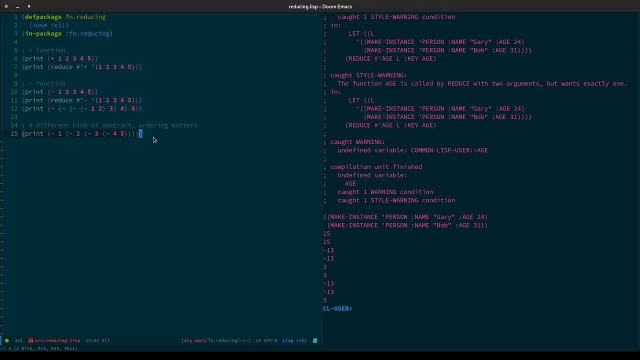 it is also 1 in the morning on a Saturday and I have been out with a friend tonight, so my logical thinking is a little bit impaired. however, I can still demonstrate this. so we have this different order of subtraction operators and if we wanted to express this in terms of reduce, we could do this using 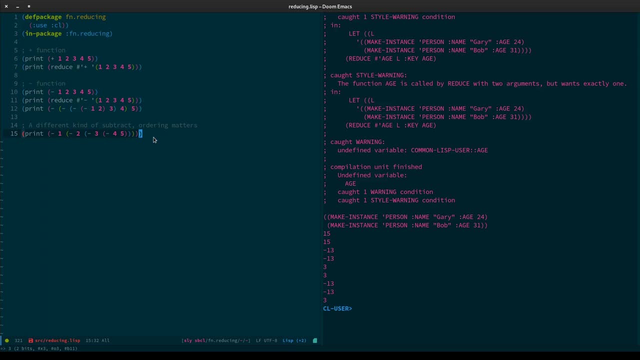 one of the key parameters that can pass in. so so this from end- we've seen this before in the other higher order functions- from end changes the order in which things are run, that's fine. so so this from end changes the order in which things are run, that's fine. 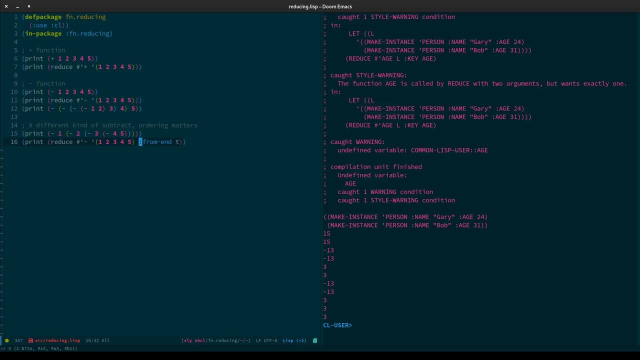 and that's where we would change the way the operators are calculated. we'd reverse the way the values are applied. so that's what from end does and that's why we get 3.. Now there's a few other things that we might want to look at. 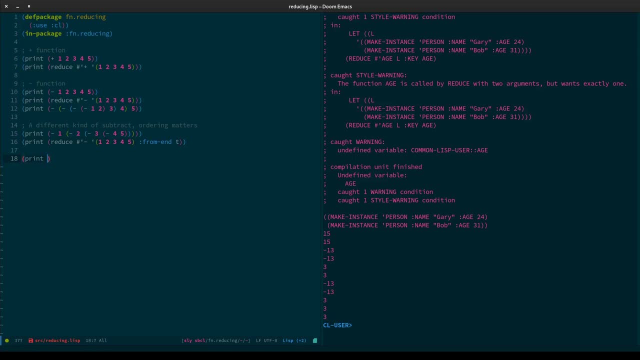 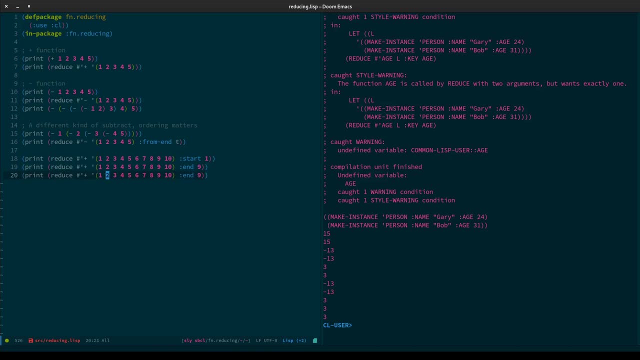 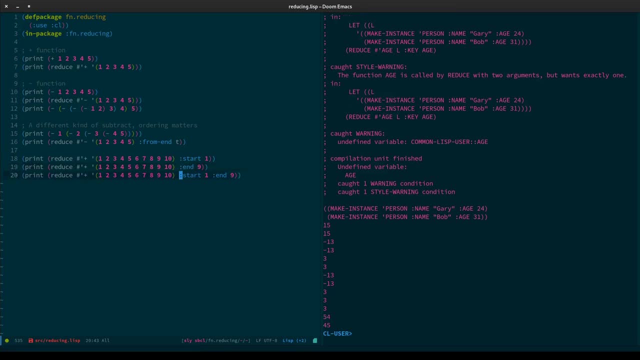 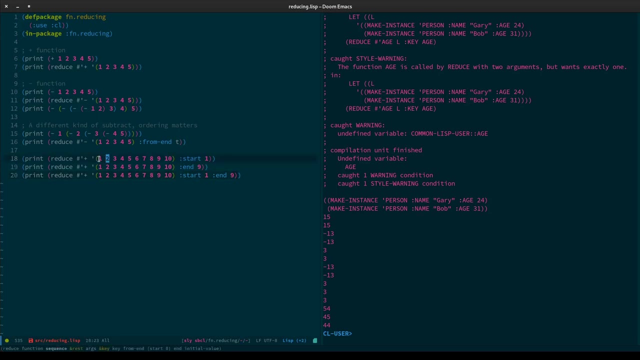 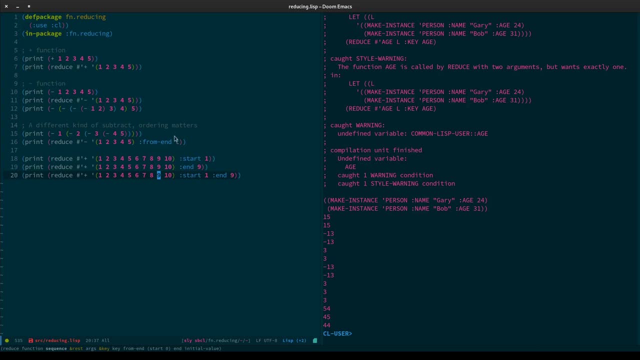 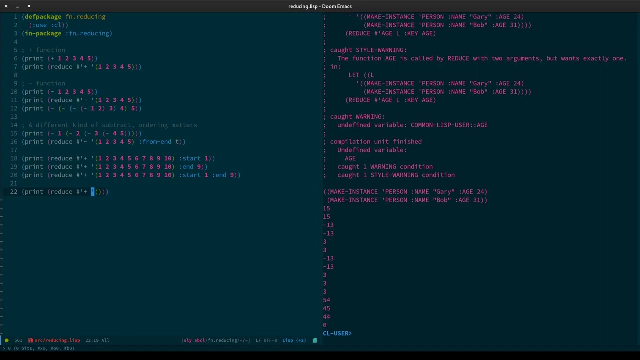 key arguments are doing, And we have this from end here. Now there's a few other. there's two other things that we want to look at. There we go. So let's say that we are using the plus operator on an empty list, which, of course, 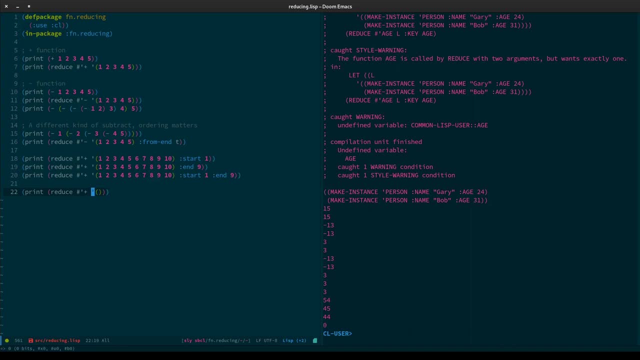 evaluates to 0.. An empty list is falsy and 0 is the falsy numeric value associated with that. So if we try and reduce that, we get 0.. Now we might want to ensure that we get some numerical value. Maybe it's the result of a calculation, maybe it's just. 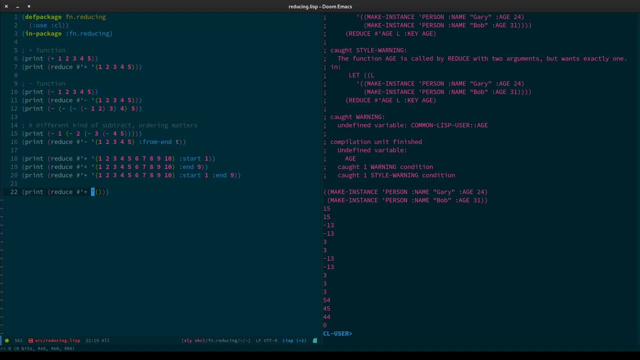 to give us some truthy value back. I don't know it depends on the implementation, But if we're going to do that, So here we're seeing, initial value of 1, so, irrespective of what the reduction did, we always start with a value of 1, so that always goes in. 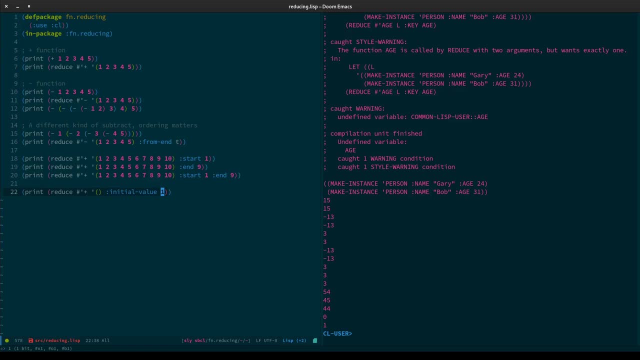 So plus 1 of 0, we still get 1.. Here, if we start with 2, we get 3, because we are adding the initial value 1 to 2.. Now it's there's some nuance to this, so let's have a look. 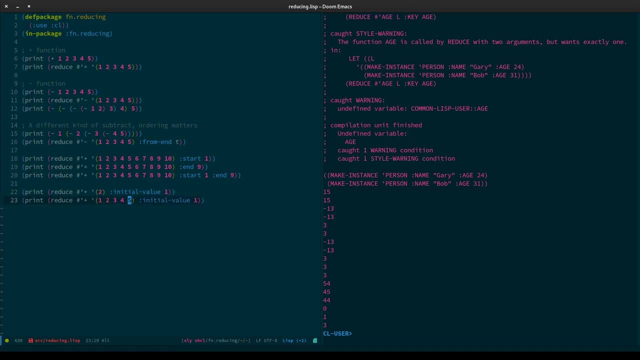 Well, we saw here where the reduction, the addition, reduction of one, two, three and five give 15.. with this initial value of 5, we would actually get 20.. So we are reducing this all down and we've got this initial value of 5,. 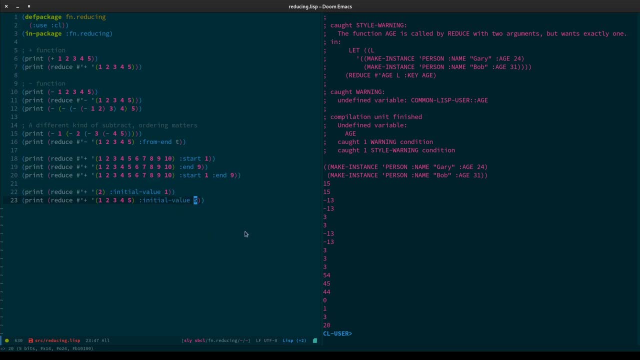 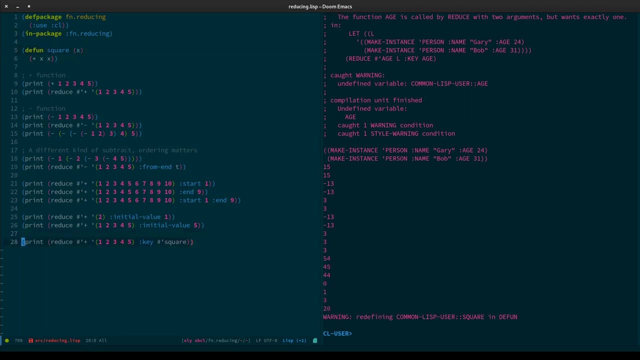 which is treated as the beginning of the list. We're going to park that for a second. Thank you, So what we have here? apparently, I defined that previously. no matter, we are going to use the reduction with the plus of 1,, 2,, 3,, 4 and 5 and we are going to use a key argument which is a function of one parameter which we've defined as square on lines 5 and 6.. 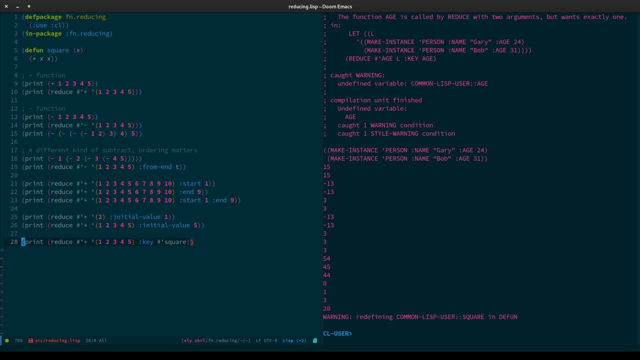 So if we evaluate that, we are going to get 55.. And that wasn't mental arithmetic, This was an example I've already prepared. So, although I struggled with the subtraction thing, please be aware that I would not have been able to compute this in my head at the best of times, just in case you were under any illusions. 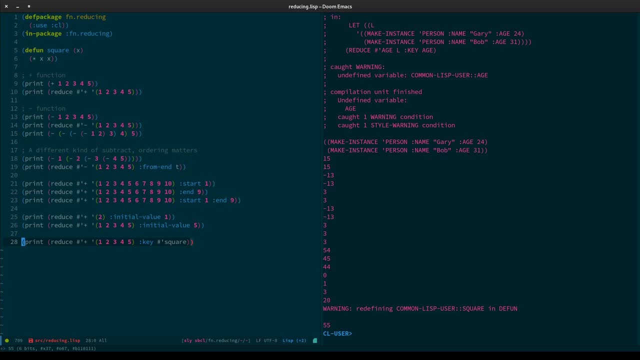 So what we're doing here is we are taking our list and we're going to add the items together, but we're going to first pass each number through this key function, which happens to be squaring them, And that's why we end up with 55 and not 15.. 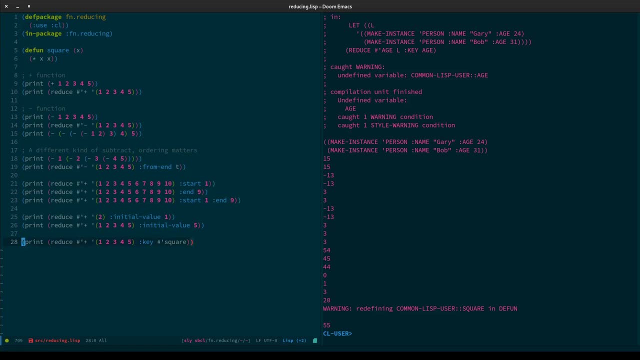 Now that Nuanced behavior I just mentioned, When we have an initial value and a key function. here it's worth noting that the initial value is not piped through the key function. So here we generate 55, but we have an initial value of 5.. 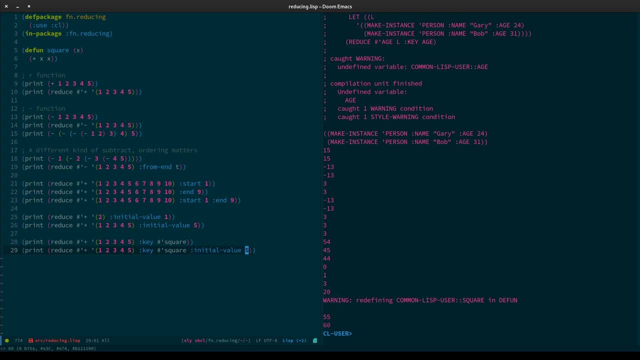 And that gives us 60.. So this proves that we have an extra 5 coming from somewhere and that is our initial value. So it's initial value plus the square of 1, which are summed together, And then that is summed to the square of 2, which is then summed to the square of 3, which is summed to the square of 4, which is summed to the square of 5.. 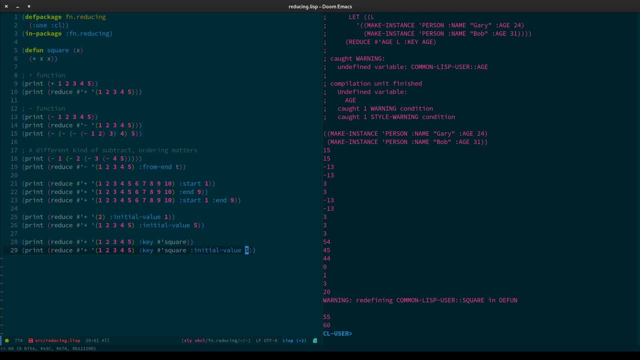 So when you're using an initial value and a key, please bear in mind that The initial value does not pass through the key function. just a gotcha. Now let's have a little bit more of an interesting example where we're just dealing purely with numbers here, but there's nothing about the reduction function. that inherently means it has to work on numbers. 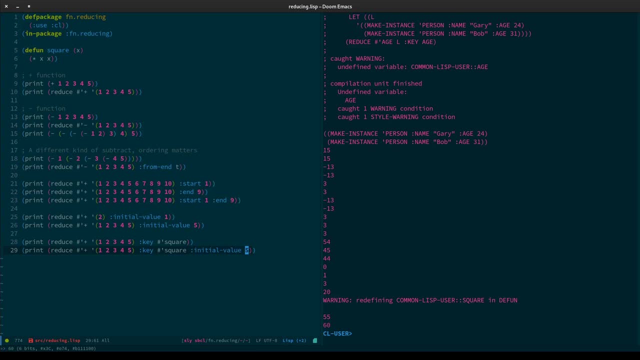 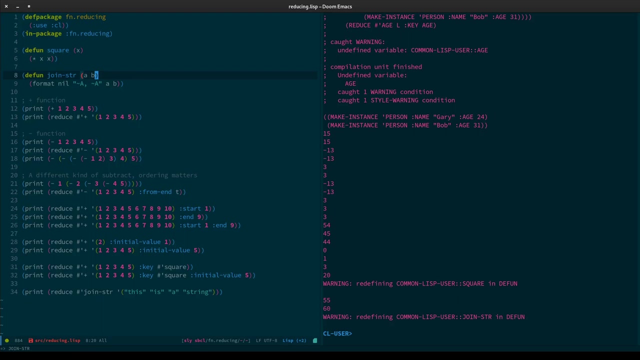 Numbers. Oh, excuse me, I am going to bed once I finish this. I am going to bed once I finish this video. Here it works. So we define this joinst function which takes an, a and a, b. So these functions must the functions that get passed into, reduce. they must take at least two parameters. 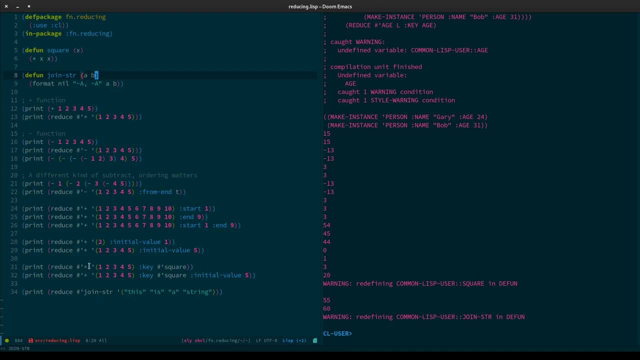 So that as they get accumulated together, So 1 and 2 go in, and then that gives a value, and that value is passed with 3, which condenses it down, and that value, that computed value of 1,, 2, and 3, gets passed in with 4, and that becomes one value. 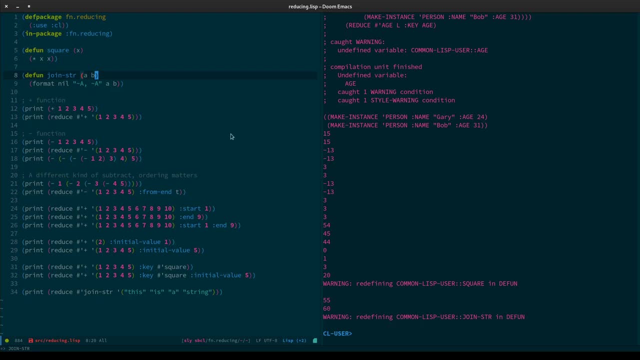 So these are being passed in in succession, with each value getting added to and just the next number passed in. So here we have a list of strings And if we evaluate this, And if we evaluate this, we actually get this. comma is comma as comma string, which is exactly what it's doing. 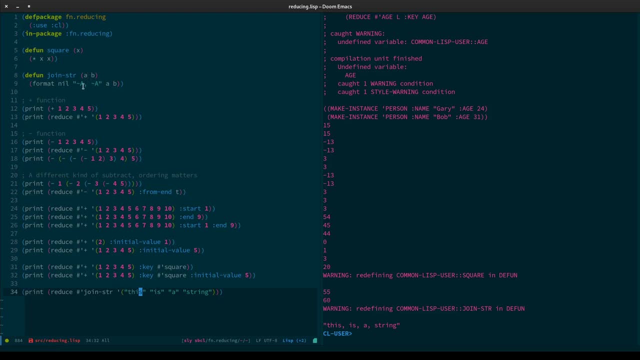 So this and is get passed in. so this goes here with a comma and is and that's returned. So this gets replaced with this comma is for the first value and that goes into a and a comes in. So we get this comma is comma, this comma is as a, and then we go comma and then b. 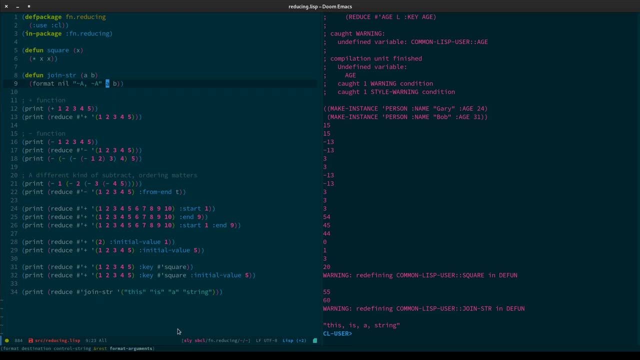 So we get this comma is comma. So we get this comma is comma a returned and that's all that replaced, And then that goes in as a and we get this comma is comma a and we do comma and then string as the b value to build that up. 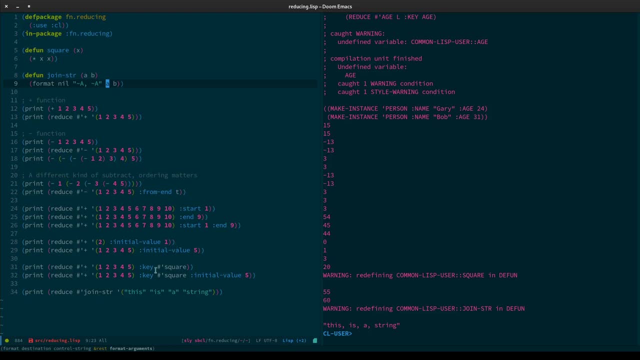 And that's what's going on here. So that's an example of how we might use strings here with a join method in a reduction function. There is a lot more that we could go into. There is a lot more that we could go into. 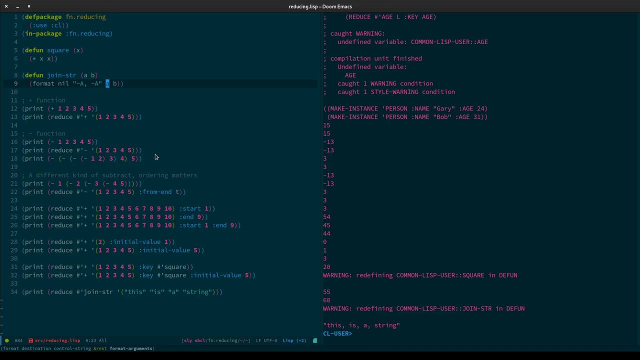 There are many examples. we could plug class into this. ultimately, I'm sure- And one of the things that I want to talk about next week- is how we combine the reduce function with the map functions that we had a look at specifically map car. 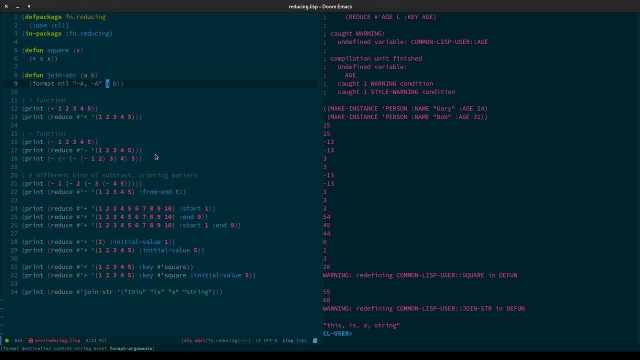 Although, given enough examples, we could use any kind of map function to plug into reduce, because map will transform our values. then we'll use reduce to combine them all together And in fact line 31 is a little bit like that, because we're using the square key function to transform elements. 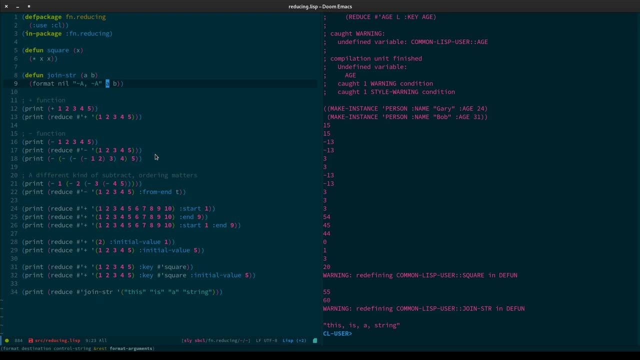 But we're not getting a list of transformed elements. We're transferring them, We're transforming them on the fly, as we get them. So it is a little bit different to line 31,. but line 31 is doing something similar that we can see. 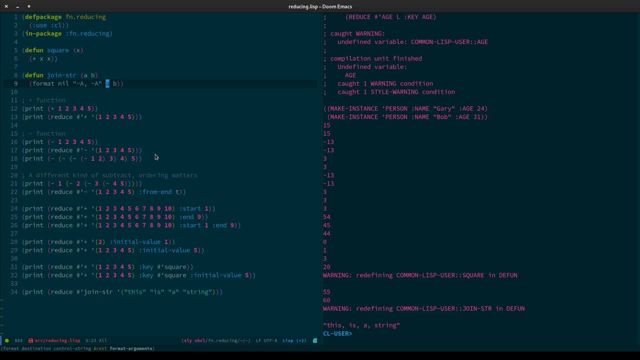 So I hope that was informative. Thank you very much for watching. I do appreciate your continued support And I can only apologize about the issues with the video earlier today. with regards to the uploading issues, I'm going to upload this now. It shouldn't take too long. 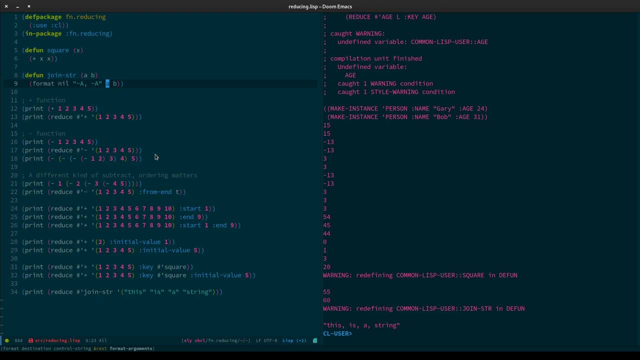 And I will see you in the next video, hopefully sometime next week, and we won't have these issues. Take care everyone.